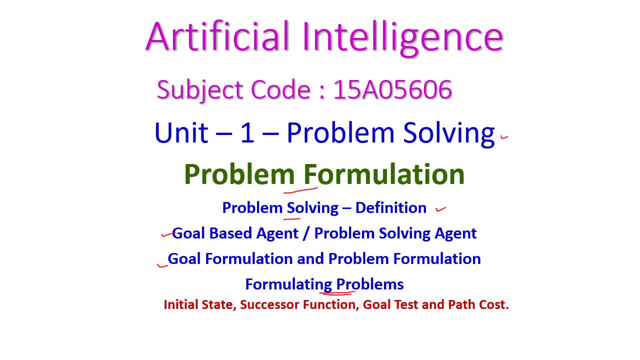 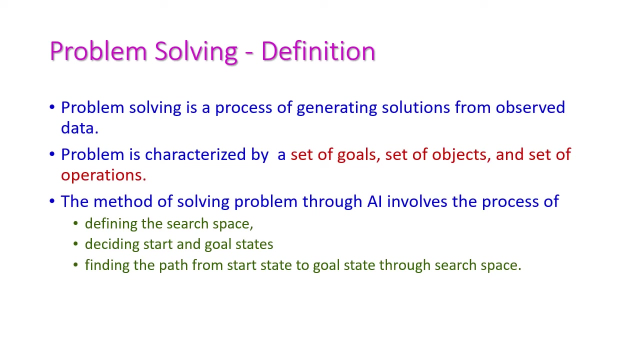 Here we are having four different components, that is, four important components are there for formulating a problem. The first one is initial state, successor function, goal test and path cast. These four are the components of formulating the problem. So these are the things we are going to see in today's class. First, let us see the definition of problem solving. Problem solving is the process of generating solutions from observed data. 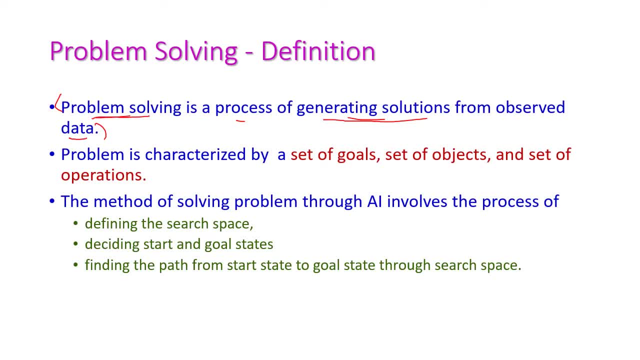 So this is called as problem solving. What is problem solving? It is a process of generating solutions from observed data. Here the problem is characterized by a set of goals, a set of objects and set of operations, That is, the operations will be performed on these objects. to reach the goals is called as problem solving. 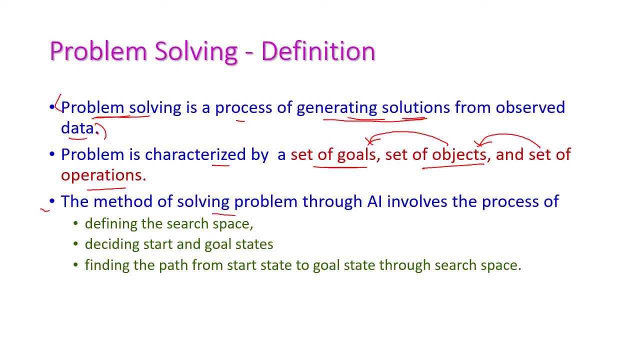 And the method of solving problem through artificial intelligence. Artificial intelligence involves the process of first defining the search space where we are going to solve the problem- defining the search space- and second one deciding start and goal state. So there should be one start state and there should be one goal state. So this is start or initial state. 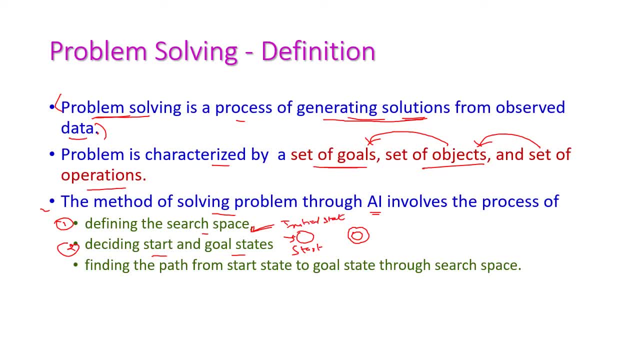 Start or initial state and this is the goal state. And third one is finding the path from start state to goal state through the search space. We need to find the path between start to goal, So this is called as the problem solving. So in this problem solving we are having three process: First one, defining the search space. and second one is deciding which is search. 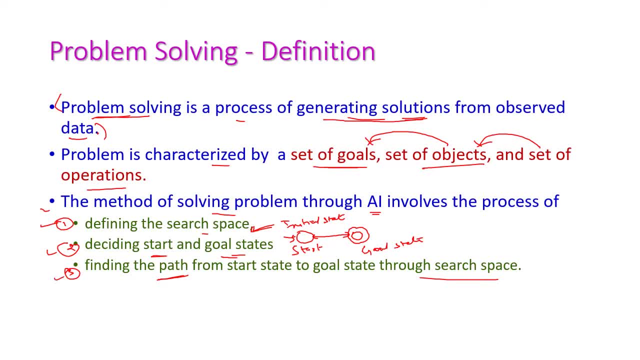 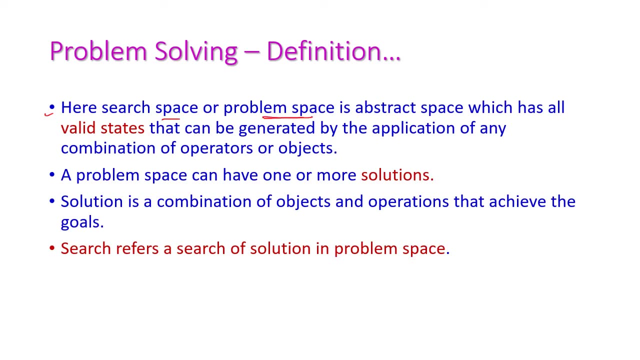 Start state and which is goal state. and third one is finding the path from start state to goal state through this search space, And here search space or problem space. Search space is nothing but problem space is abstract space which has a valid states, Which has valid states that can be generated by. 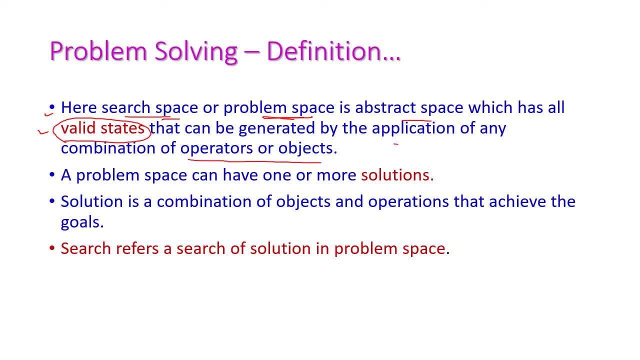 The application of any combination of operators or objects. So by using this we can create the valid state Here. the search space is otherwise called as problem space. that is nothing but agent world, which is otherwise called as our environment. That is agent environment, Okay. 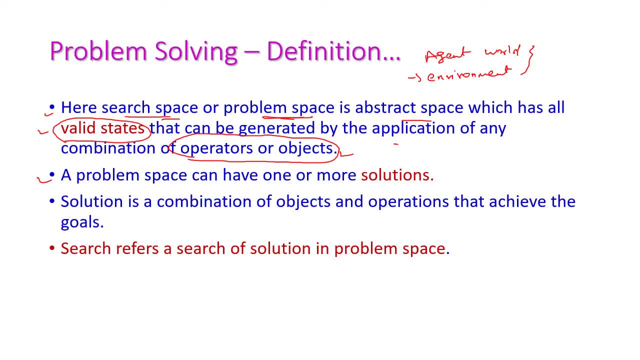 And The, The problem space, can have one or more solutions, So sometimes a problem may have more than one solution, but we need to find the optimal solution. Okay, And solution is the combination of objects and operations that achieve the goal. Okay, 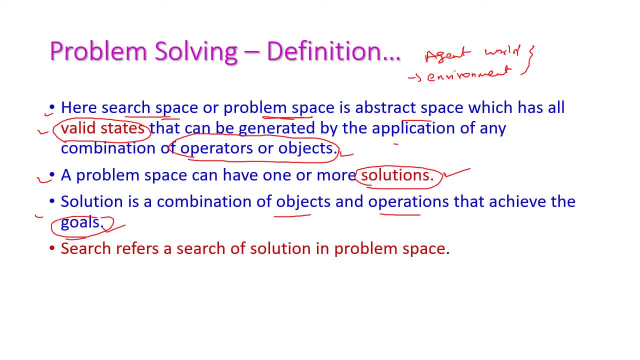 Solution is nothing but the combination of objects and the corresponding operations. Okay, Those are helpful to achieve. this goal Is called a solution And search refers a search of solution in the problem space. What is mean by search? Search is nothing but to find the solution from the problem space, from starting state to goal state. 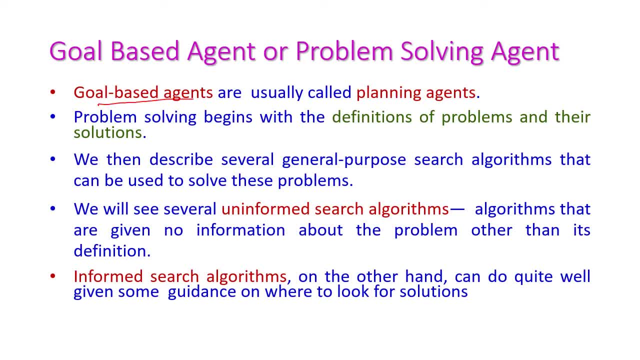 And here this is the goal based agent, which is otherwise called as planning agent. Okay, And problem solving begins with the definition of problem And their solutions. So for solving any problem, we should have the definition of problem. The definition of problem should be clear. 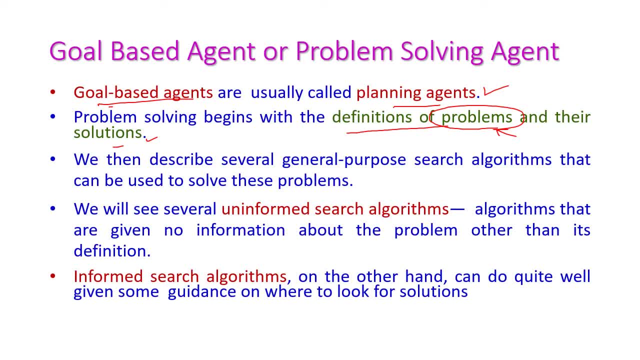 Okay, If the problem is correct, then definitely, we will have the solution for that And we can describe several general purpose search algorithms that can be used to solve these problems. Okay, So, by using this goal based agent or problem solving, Okay, And we will see several uninformed search algorithms in this unit. 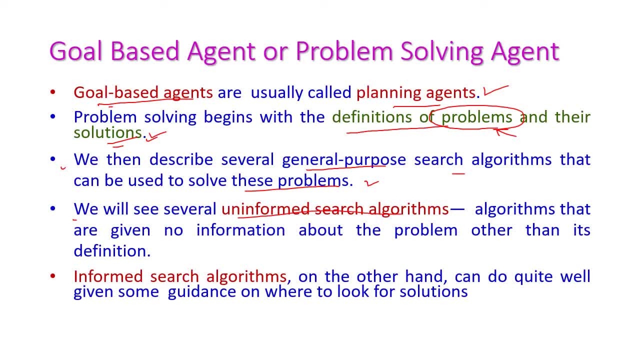 Okay, Several uninformed searching algorithms. Uninformed searching means the algorithm that have no information, that is, no additional information about the problem other than its definition. We can get that information only from the problem definitions. Apart from that, we don't have any other information. 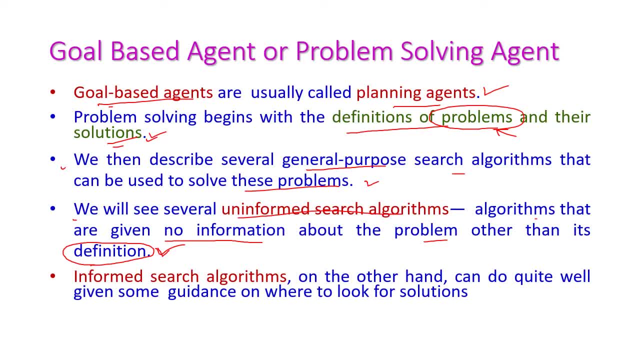 And those problems are called as uninformed search algorithms. Uninformed search algorithms- Okay, Example for this uninformed search algorithm are: breath first search, depth first search, uniform cost search and depth limited search, etc. So these are all example for uninformed search algorithm. 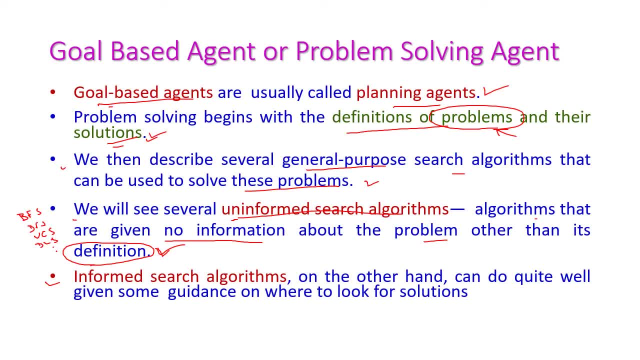 So after that we are going to see the informed search algorithms And here There are some guidance on where look for solutions. So by using some guidance we can easily find the solutions. So these are called as informed search algorithms. Okay, The example for this informed search algorithms are greedy best first search algorithm and A star algorithm, AO star algorithm and etc. 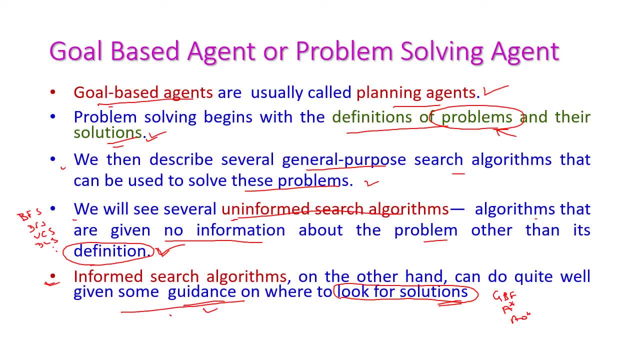 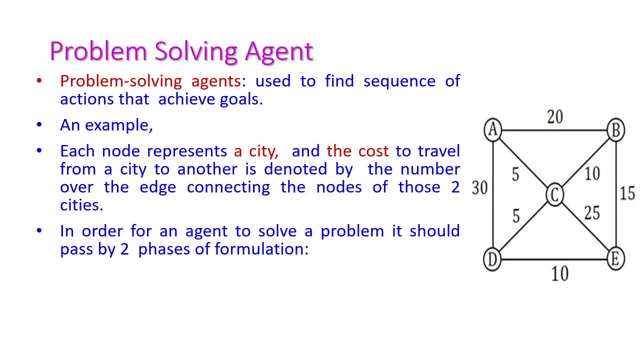 So these are all example for this. So these are all example for this: informed search algorithms. Uninformed search algorithm means, apart from problem definition, we are having some other information to reach the solution. Okay, So that is called as informed search algorithms. 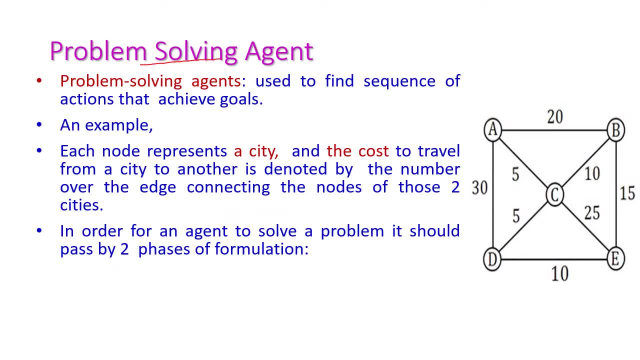 And next we will see some more detail about this problem solving agent. Right, It is used to find the sequence of actions that achieve goals. What is the purpose of problem solving agent? The problem solving agent is used to find the sequence of actions. 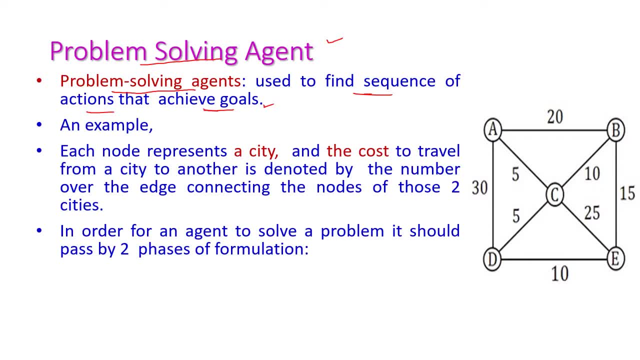 What are the actions will be there to reach the goal? Okay, That is used to decide by this problem solving agent. Let us see one example for this. So here we are having one graph. Okay, This graph represent the cities. So A is the start city. 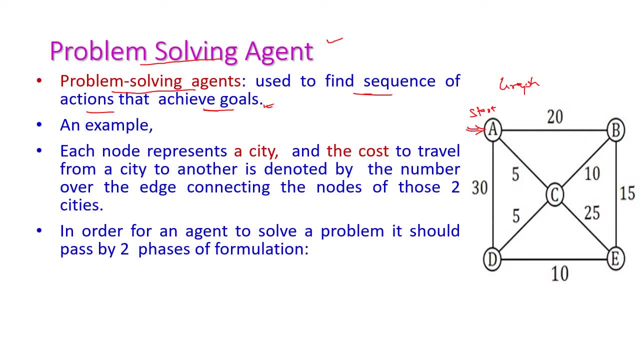 Start city Starting state. We are currently in A And we are having some other cities also. Okay, B, C, D, E are cities And this is our goal. We are going to reach this E. Okay, How do we reach this E? 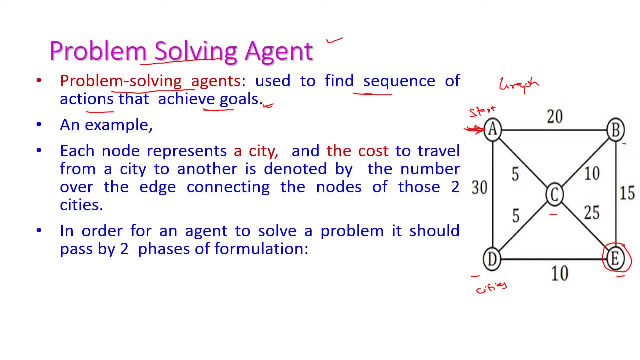 What is our problem? Okay, Here the node represent city, Which are? the nodes? A, B, C, D, E are represent city And the cost. This is important, The cost to travel from a city to another city, denoted by numbers, 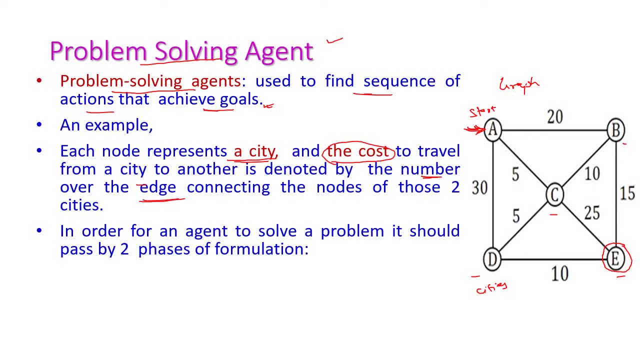 Denoted by numbers over the edge. Okay, So the edge is having the cost. Okay, The cost for travelling from A to B, For example, The cost is 20.. This may be 20 km Right And in order for an agent. 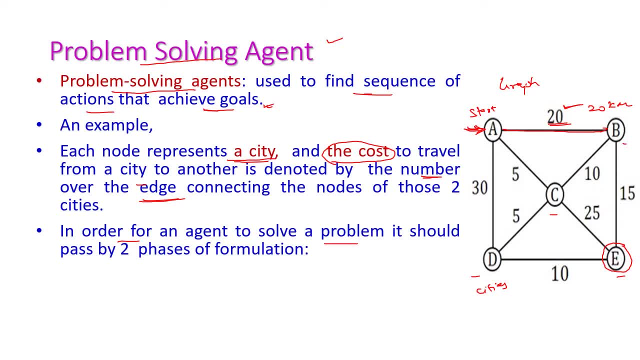 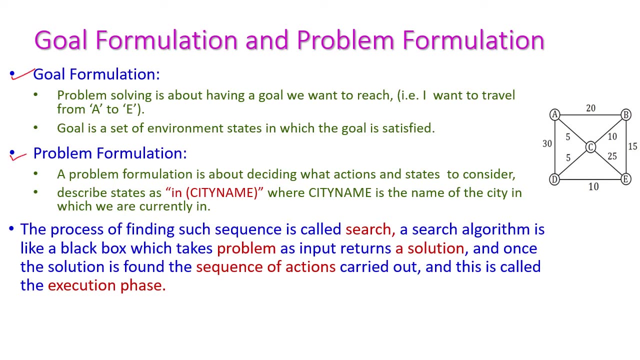 So to solve a problem It should pass by two phases of formulation. Okay, Let us see what are those two phases of formulation. The first one is goal formulation And second one is problem formulation. Okay, Goal formulation, That means the problem solving is about having a goal. 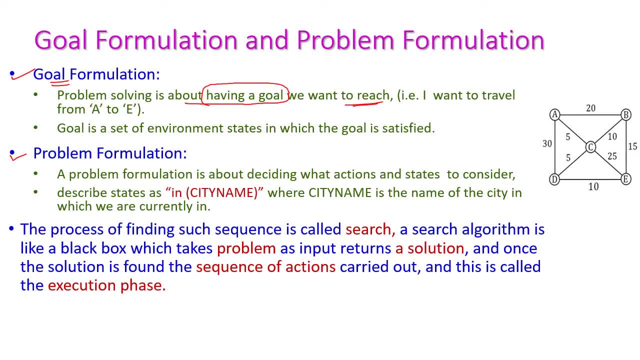 Having a goal we want to reach. Initially, we are in starting state And this is our goal state, So we need to reach this goal state. Okay, I want to travel from A to E. How do I travel? Which path I am going to choose? 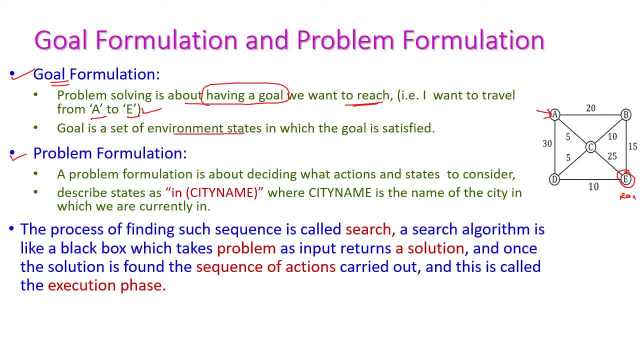 Okay, And goal is a set of environment states In which goal is satisfied. Okay, So goal is having some constraints. We need to satisfy that constraints in all the states And which states is satisfied. that is called as goal Right. And next one is problem formulation. 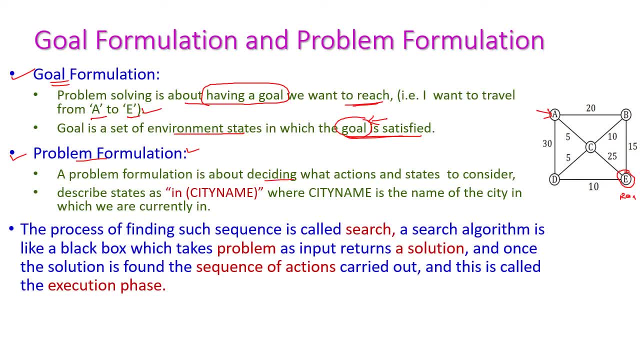 Problem formulation is about deciding what actions and states to consider. Okay, Which action is to apply to reach the next state? Okay, So describe the state in city name. Okay, Currently we are in this particular city name, For example, in A. Currently I am in A. 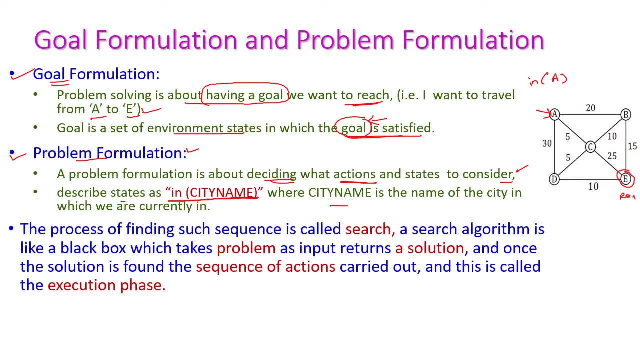 Okay, Where city name is name of the city in which we are currently in. Currently, we are in city A, So from this A we need to go to B C, go to b c, d, r, current, current. finally, we need to reach e and the process of finding search. 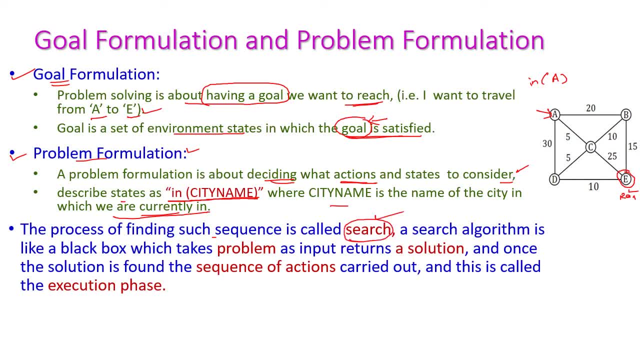 sequence is called as search. okay, in what sequence we are doing all the actions? that is called as search and search algorithm is a black box. we don't know anything inside the box and it takes problem as input and returns a solution. okay, so input, this is the search. we don't know anything. 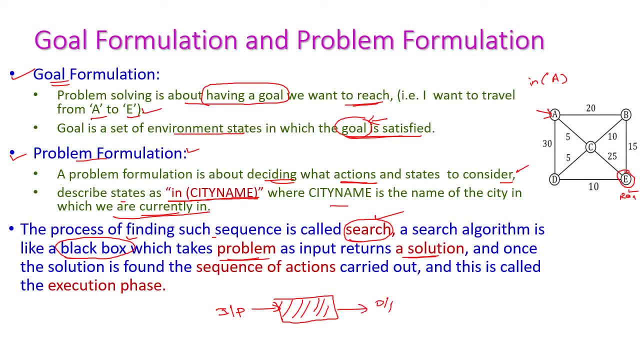 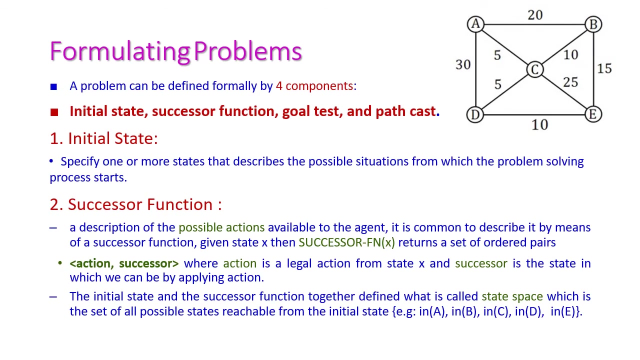 in this and it will give output. input is problem, output is solution. right, once the solution is found, the sequence of action carried out and it is called as execution phase. okay, so this is execution phase. the next one is formulating problems. the problem can be formally four components. four components: 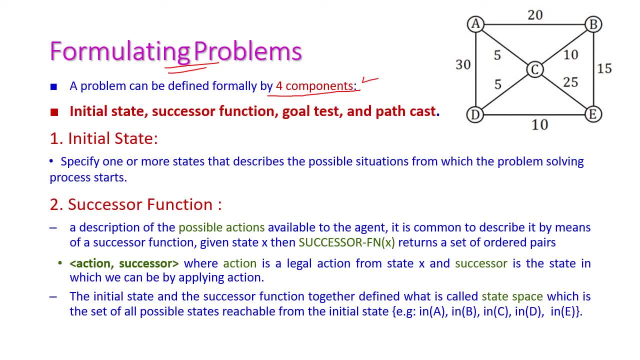 are very important for formulating any problem. the first component is initial state, second one is successor function, third one is initial state, third one is goal test and the last one is path cost. all the four components are very important for formulating any problem. first one is the initial state. okay, so here the initial state. 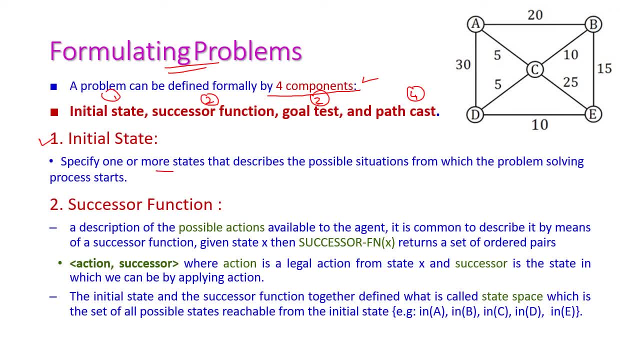 is to specify one or more states that describe the possible situation from which the problem solving process starts. that is the starting point of the problem solving is called as initial state. in our problem the initial state is a okay initial state right and next one is successor function. 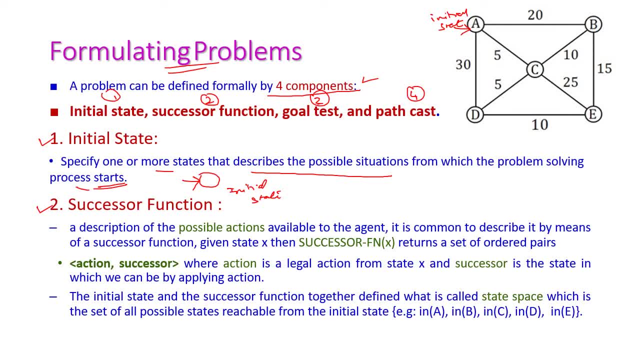 successor function is description of possible actions available to the agent. okay, what are the possible actions available to the agent is common to describe by means of successor function. so this is the first part of the problem solving process: Successor function. by using the successor function, We can describe what action to be selected. 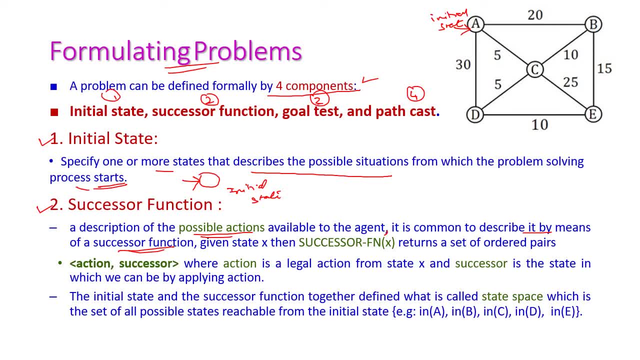 if so, what successor State we will reach then? this is the successor function. Okay, returns a set of ordered pairs: action comma successor. Action comma successor, which this successor means. successor state- Okay, successor state, neighboring state where action is legal action from the state X and successor is state in which we can. 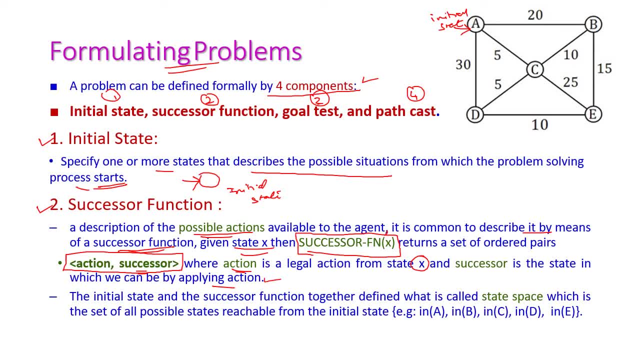 We can be applying action, The initial state and successor function together, Defined what is called as state space. Okay, here we are having five different state space, which is a set of all possible states reachable from initial state to the final state. Okay, here, what are the possible states we are having in our problem? 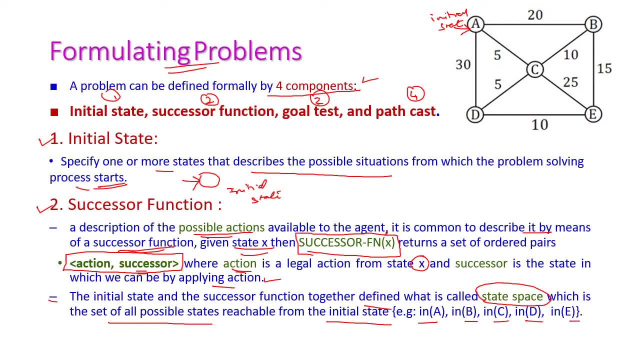 A, B, C, D, E. all the states will be reachable from this a only. Okay, from a we can reach all the states. So we can reach this B, We can go to this D, We can go to this E. from C We can go to the E also. 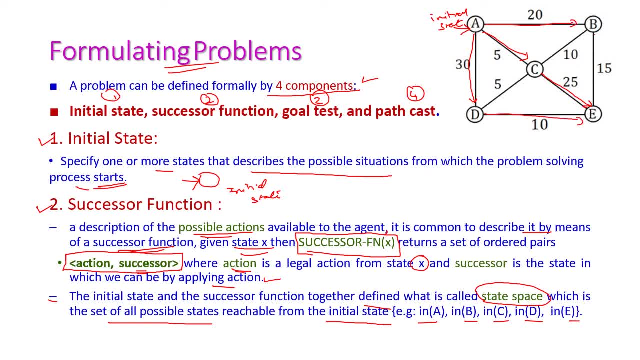 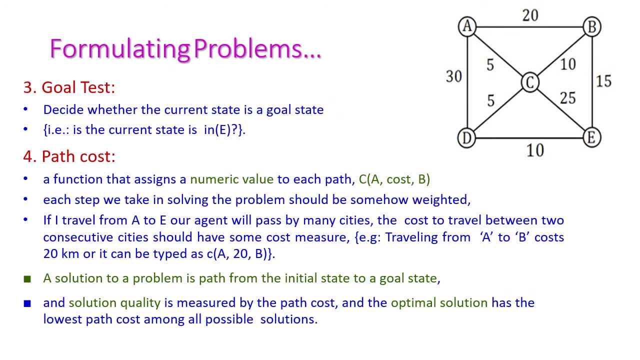 Okay, from D also, we can reach e. from b also, we can reach this e. okay. so this is called as formulating problem, that is, successor function. next one is. next one is gold test. right, gold test decide whether the current state is gold state or not, so this is called as gold test, gold test. so for any problem, 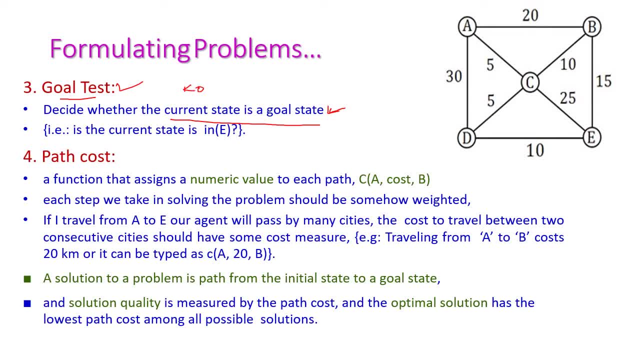 we should know which is good: knowledge about the goal, knowledge about the goal. so we should know the knowledge about goal previously. then only we can test whether the successor node is gold node or not. okay, so for every state we need to test whether successful or not, The current state is E or not. 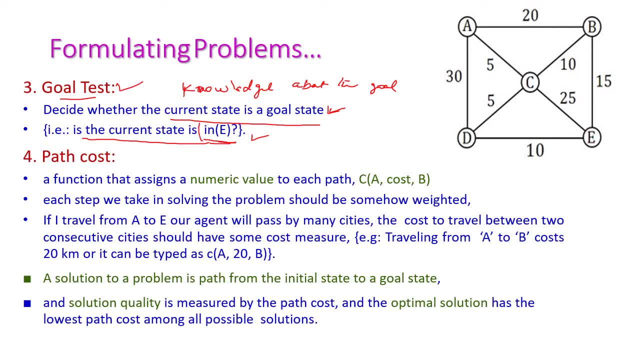 Okay, so we should know the state E is the goal state And next one is path cast. That is, path cast is nothing but a numeric value to each path. Okay, the formula for this is cast, Cast of A is current state, cast and B is the successor state. 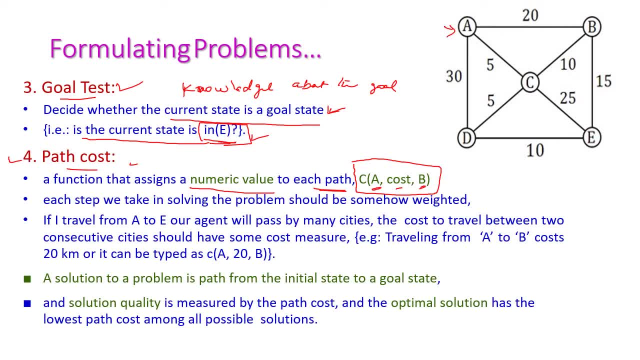 Okay, so A is the current state and B is the successor state. In between, what is the cast? Each step we can take is solving The problem should be somehow weighted. Okay, all the edges should have its own weight. Okay, when we apply this particular action, we need to pay this much cast right to reach the next state. 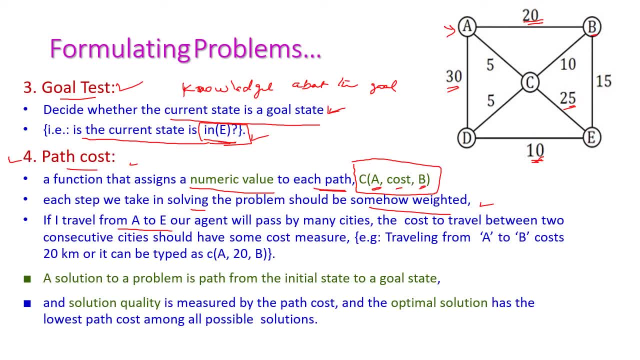 So if I travel from A to E, our agent will pass many cities and the cost to travel between two consecutive cities should have some cost measure. Example: suppose I am going to travel from city A to city B. the cost is 20 kilometer. 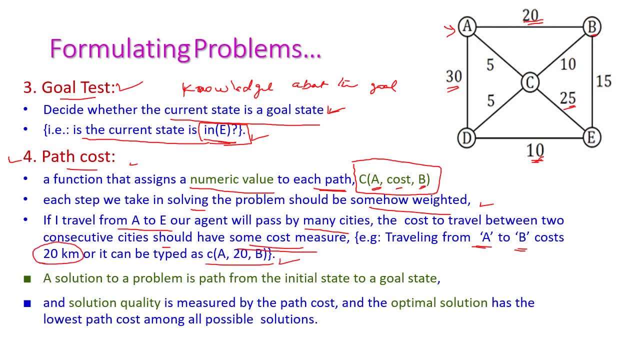 Or we can return this as in this form: Okay, C. C means cost. Cost of A to B is 20.. The solution to a problem is path from initial state to goal state. What is the path from initial state to goal state? 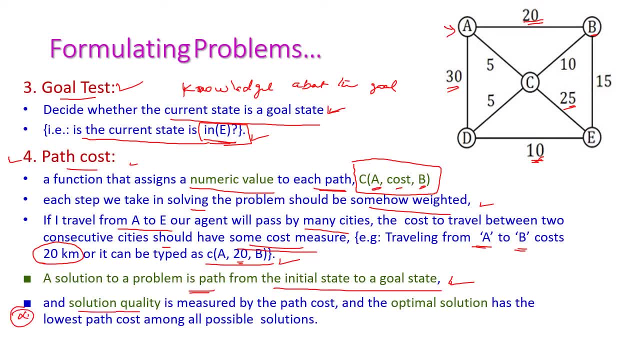 And this is important. Okay, the solution quality. The solution quality is measured by path cast And the optimal solution. The optimal solution is the lowest path cast among all possible solutions. So if the optimal solution should have minimum path cast, Minimum path cast among all the possible solutions, right. 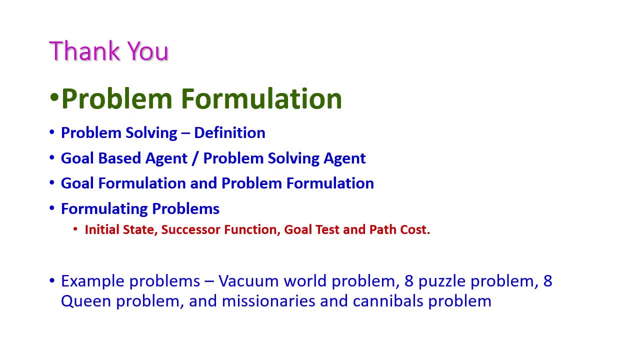 Up to this we have seen the problem formulation, that is, introduction about this problem formulation. In this introduction class we have seen the definition: goal based agent and problem solving agent, goal formulation and problem formulation And formulating problems. under this we have seen the four important components, that is, initial state, successor function, goal test and path cast.